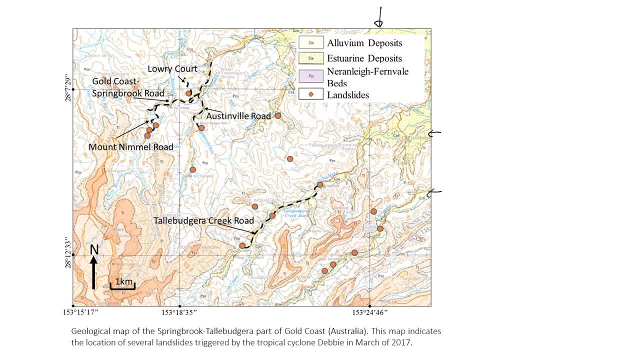 It will represent the type of rocks or soil And if you don't know which exactly it is, so we can look at the legend. So this is an important part and this is called legend. So legend gives you explanation on the color And it shows what deposits in the soil or rock belongs to each color. 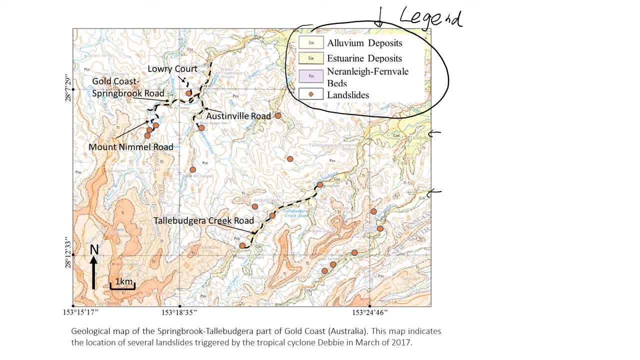 Another important thing about this map is the scale, Because we would like to know the distance from the land From this point to this point, To know that we're going to use the scale, And scale in this case is given as one kilometer. So this much on the map will give you one kilometer in real life in that area. So sometimes you will see that there are maps. their scale goes like one over 250,000. 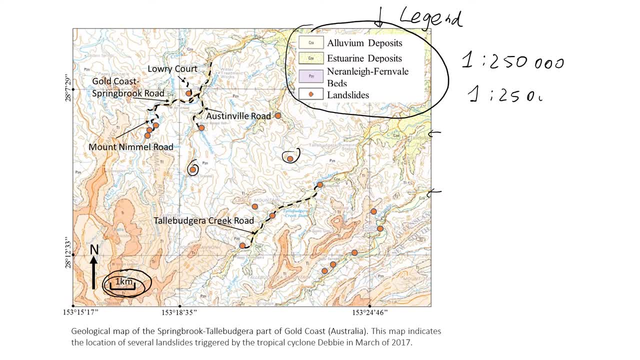 Sometimes there is maps- one over 25,000. So how do we read this one? So the easiest way to read this map, and the way that I do, is I just remove two zeros from the right end And it will give me a scale: one centimeter It's equal to. in the first case, it will be 2500 meters. 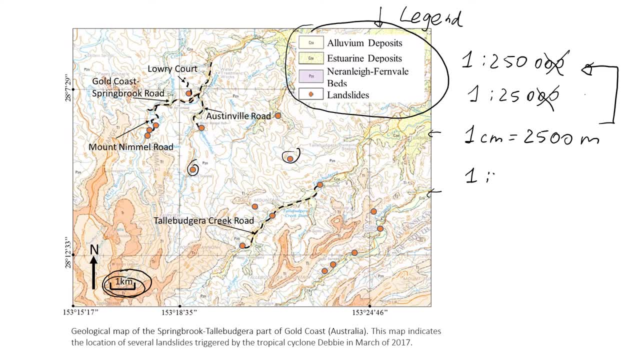 And in the second case is going to be one centimeter equal to 250 minutes. Why do we have different scales? It actually depends on what kind of investigation we would like to do. For larger areas, for general maps, we typically have a larger scale, like this: 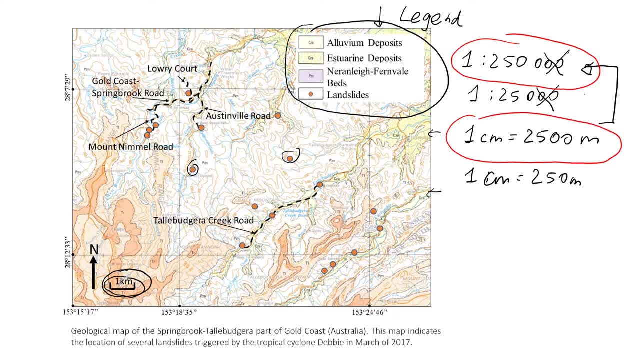 So this is to cover larger areas For some specific sites. when we do a detailed investigation, we will have a larger scale like this investigation. we would like to have more precise map with a scale like, for example, like this one: one centimeter, 250 meters. okay, let's see. what else do we have here on this map? so this map was about 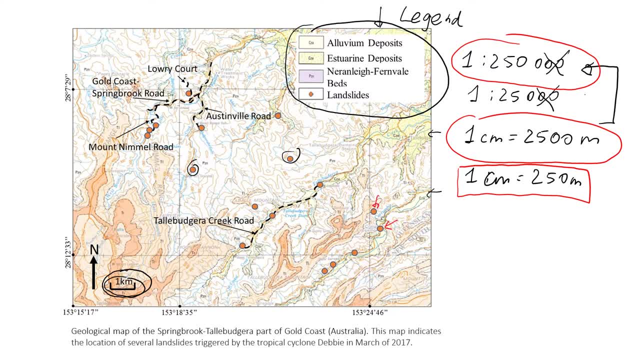 landslides and you will see this is location of landslides. there have been lots of landslides in that area and some of them just triggered by rainfall, some and and I think it shows north and south- there is one important part that is missing and which doesn't make this map very valuable, and 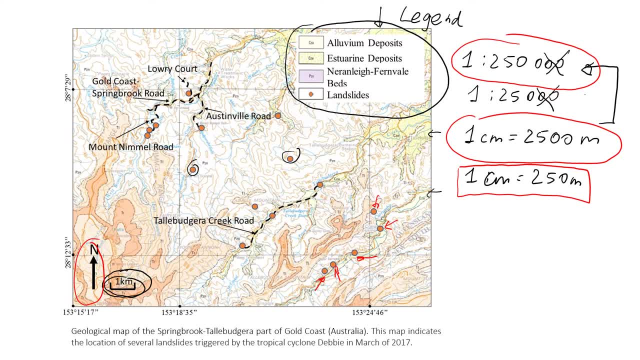 if you look at the map, you will see that there is different types of rock and soil on the surface, but we don't know what that is because we only see levels of lava on the surface and this is in the what material is underneath the surface. so if we go, 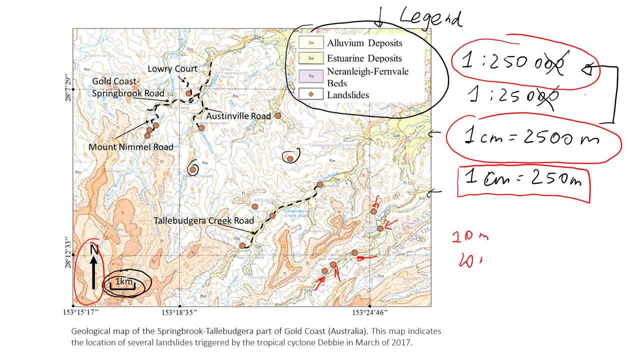 like maybe 10 meters deep or 20 meters deep. we don't know what is in there. so the part that this map is missing is called cross section. cross section would show you the location of different soil and rock layers underneath the surface, and this is what a good geological map should always come. 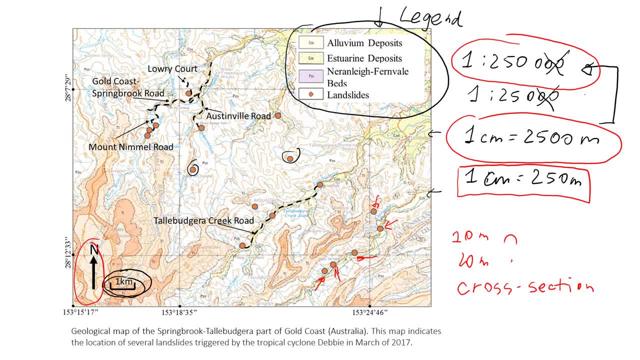 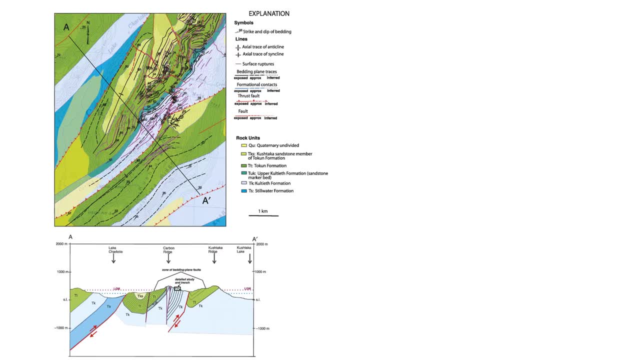 up with. and now let's look at the second map. so the second map it's some area. to be honest, i don't know where the area is, but we're just going to look at the map and see what is presented in here. so again, you will see that it has. 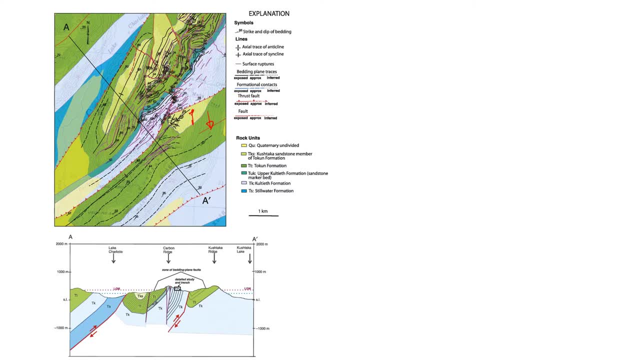 different colors and these different colors- green, yellow, blue- they all explain in the legend. so it says explanation. some people call it legends. so you see there's explanation about the color. it represents a different geological units, mostly in this case rock units. we have different rocks right on the 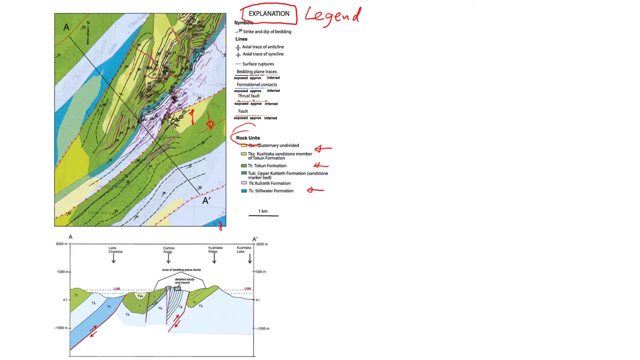 surface. another thing that is important: it's folds. so typically they're shown on such geological maps as a line and it's going to be a red line, like you see one red line here. so this is the fold. this is another fold. folds are very important, especially when we do site. 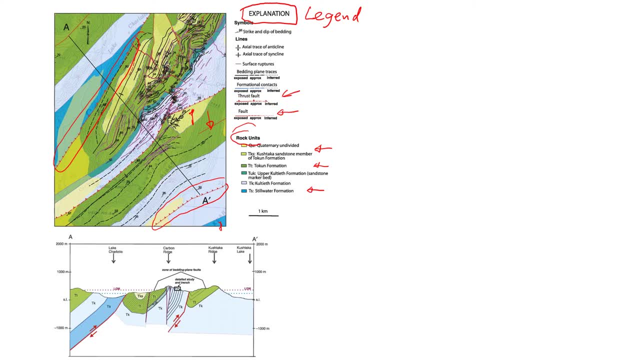 investigation. we need to identify these folds because falls typically create very fractured and weathered rock. typically, falls are associated with some soil movements as well, so that's not really good engineering foundation defaults and also it shows some bearing planes strikes, and deep, if you don't know what beating planes. 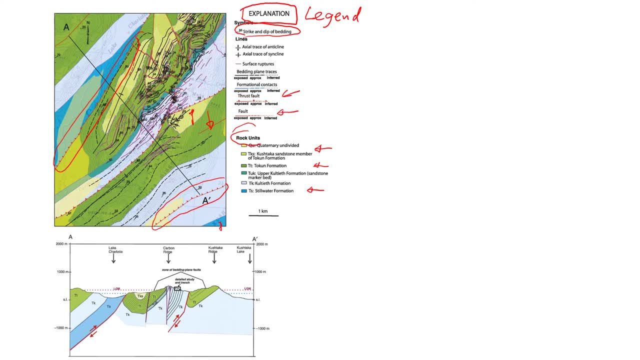 means please watch my video on bearing planes and it also, given the scale, and we can see that the, we can see that the, the, the, the, the, a dash here. so, um, i will have another video, how to draw cross section. i just want to explain that cross. 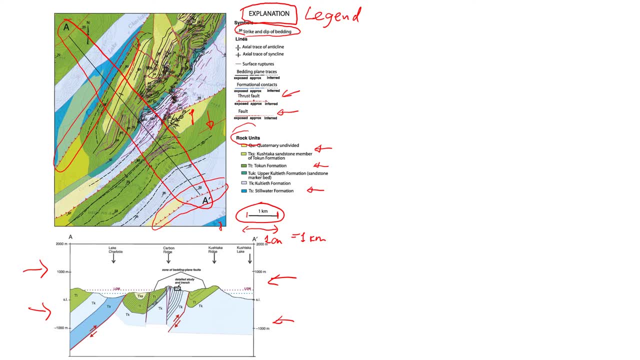 section will show you the material underneath the surface. so typically for cross section we need to drill a few more holes and all the data about geology underneath the surface comes from those bore holes. so you will see that when we look at the cross section, what is underneath the surface up to 1000 meters? 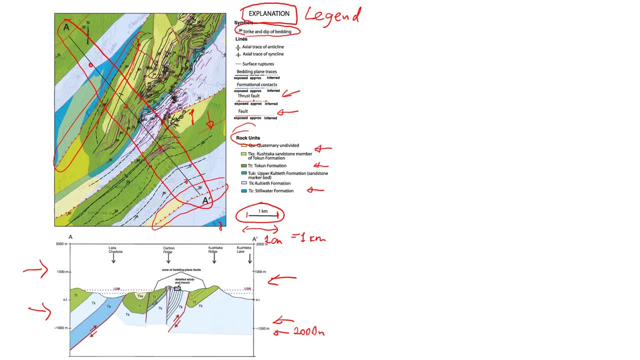 deep, so this is thousand meters. we have a very good understanding about the type of frogs that are present and how they are placed against each other. you will see that we have layers of different drugs and they're deep at some angle, steep angles. so here we also see there is this fault goes in this direction.